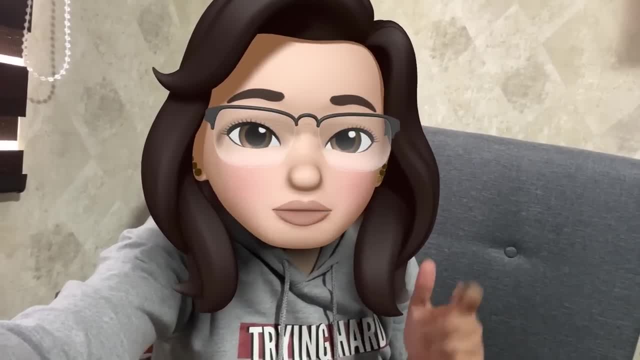 So this is part one. We're going to talk about understanding sentences and what that means, And before we jump into that, just a quick little plug: If you're interested to get the reviewers that I made join the online or live review. 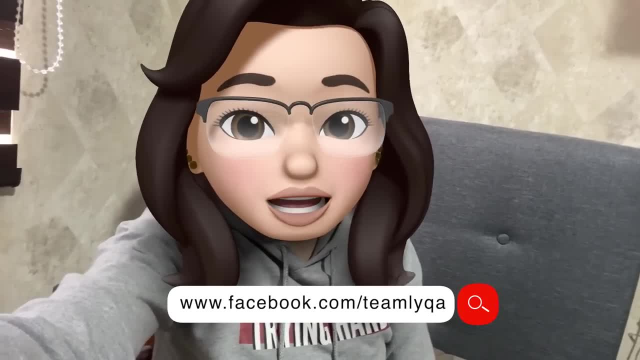 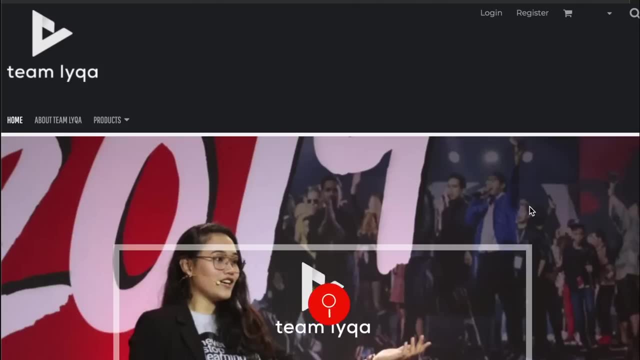 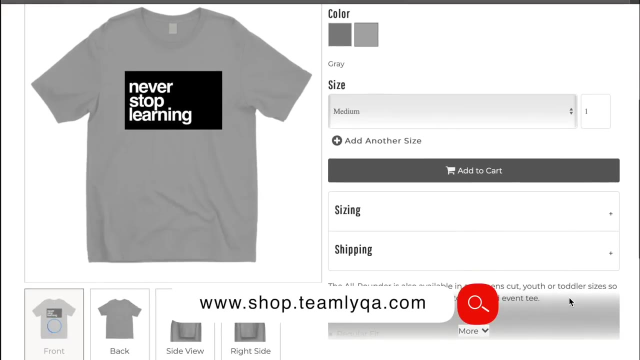 You can go to wwwfacebookcom slash Team Laika for more information, And this is our trying hard hoodie. We also have a shirt, caps and merch shop at shopteamlaikacom. All the links are in the description box below. Okay, and now that we have that out of the way, 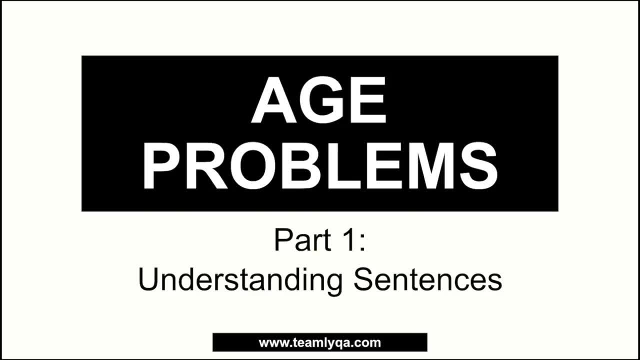 I'm going to jump right into it. I'll see you in a bit, All right, so this is part one of our comprehensive series on age problems. We're going to talk about understanding sentences, Basically what it means if, say, a person is older than you. 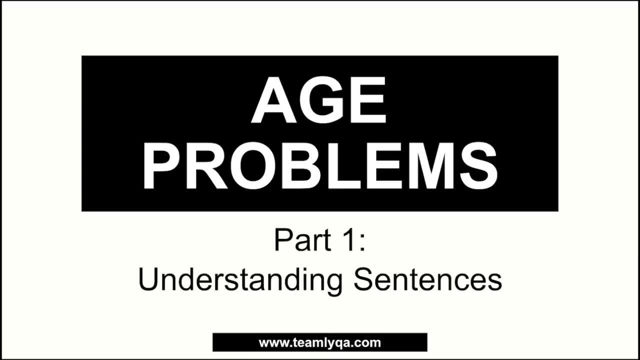 than this person. a person is four times as old as this person- and how they convert into an equation or how you can understand them enough so you can draw your table. I already have older videos on age problems, but I didn't stop it like this, and that is the reason why I'm making this. 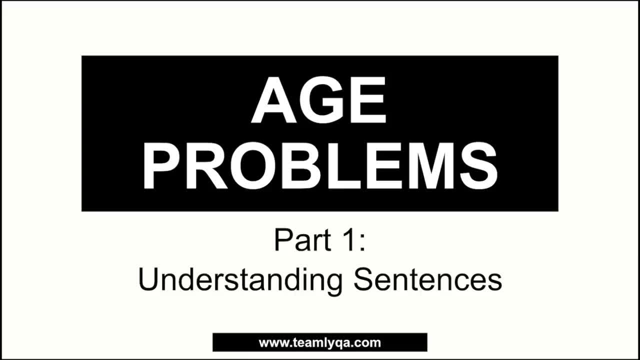 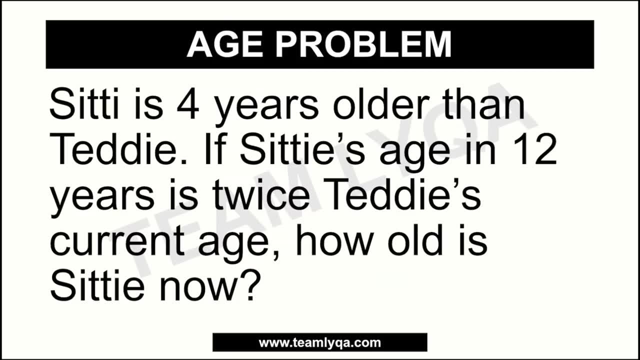 series. Hopefully, after this entire series that you will watch, you will understand it better. Now, first problem that we encounter when we encounter a problem like this is: kung gaano siya ka-complicated pakinggan. So sabi si T is four years older than Teddy, If T is aged in 12 years. 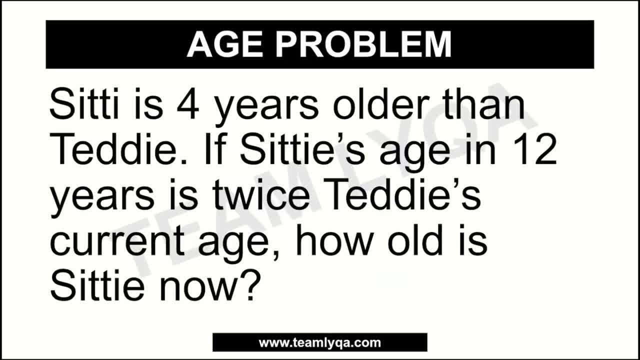 is twice Teddy's current age. How old is T now? So ang dami masyadong factors na nagka-come into play and hindi natin sila masyadong maintindihan agad, kasi nga ang daming nangyayari So kailangan. 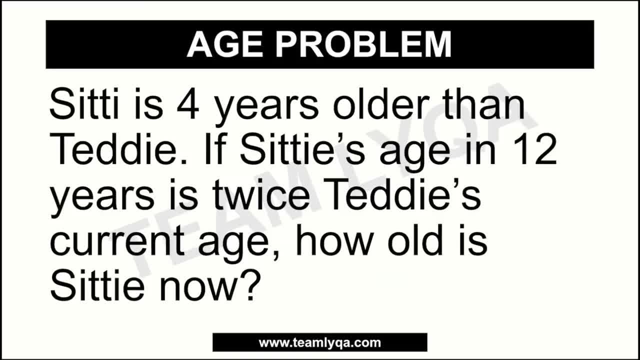 natin siyang himayin, isa-isayin natin sila. Now, ang first step doon is breaking it down into smaller pieces. So the first step is to break it down into smaller pieces. So the first step is to. 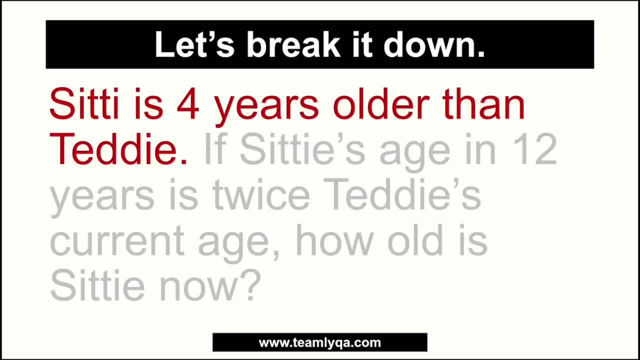 that you have to take note of is this statement right here: Sabi si T is four years older than Teddy, So kung ito munang statement na, yan ang hihimayin natin, yan munang pag-uusapan natin. 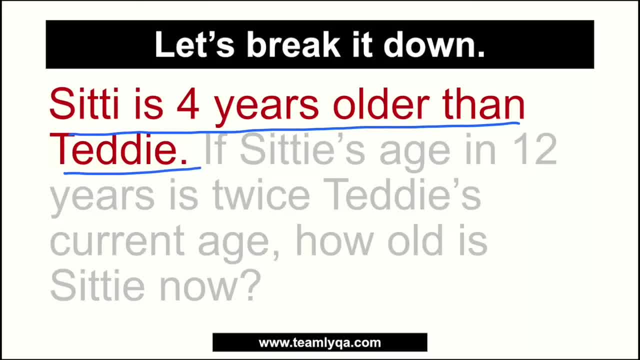 anong ibig sabihin yan, And a lot of people have trouble with finding out kung sino ba talagang mas matanda. sino ang ilalagyan ko ng plus four, ima minus four ko ba yan? ano ang gagawin ko? 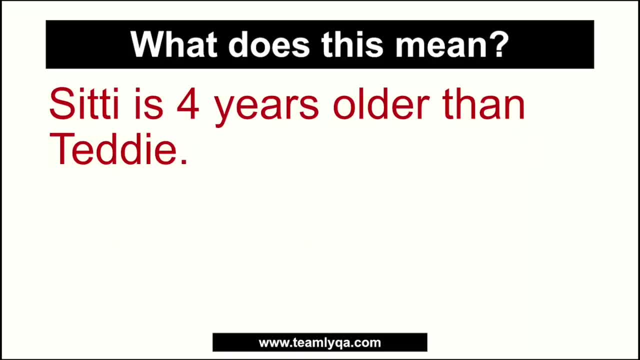 So anong gagawin natin? Tingnan muna natin yung sentence. Sabi si T is four years older than Teddy. Now the best thing about us being bilingual as Filipinos is: pwede mo itong tagalugin or translate into your heart language, Magsasabit? 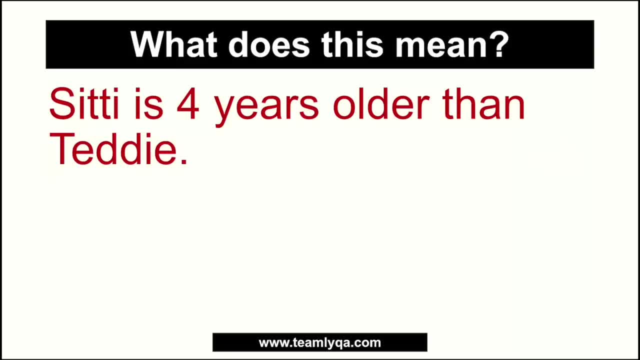 yung heart language, ibig sabihin yung first language ninyo. Ano ang language na una ninyong natutunan, And pag nagawa mo yun, mas maiintindihan mo yung problem. For example, sabi dito: 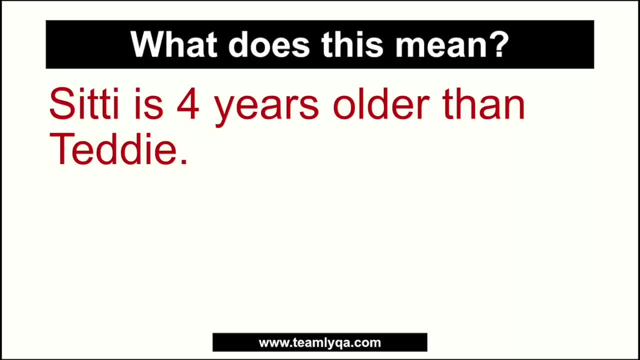 si T is four years older than Teddy. Sa Tagalog si T daw ay apat na taong mas matanda kesa kay Teddy. Kasi ang first question is: sino ba talaga ang mas matanda, Si T o si Teddy? Now again, 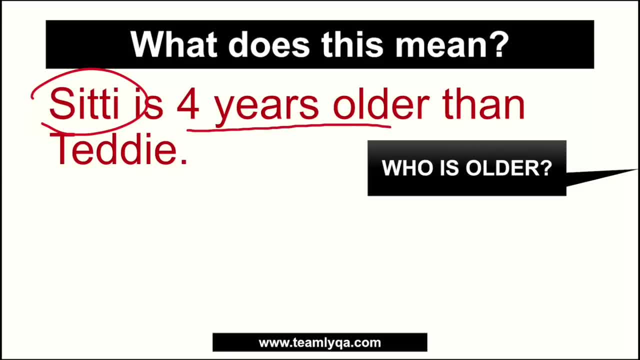 yung age daw ni si T ay four years na mas matanda kesa kay Teddy Sinong older, Ang older is si T. Okay, Si T is older, Kasi four years nga siya mas matanda kesa kay Teddy, So ibig. 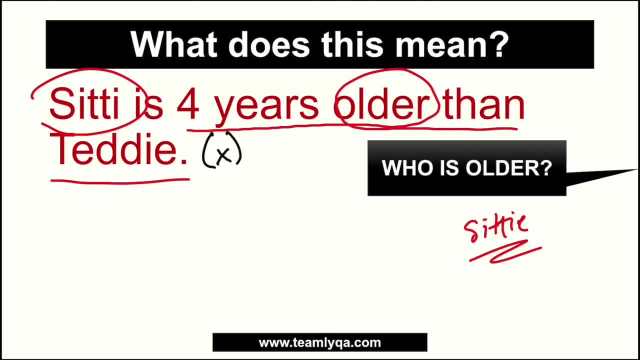 sabihin nun, kung si T ang X sa problem na ito, para malaman natin yung age ni si T? that would be: yung age ni si T ay four years na mas matanda, kesa kay Teddy. So ibig sabihin nun: 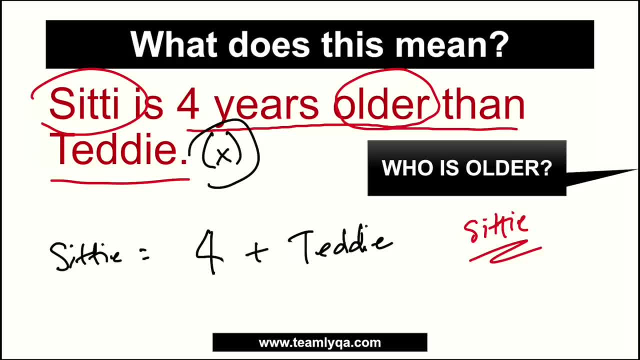 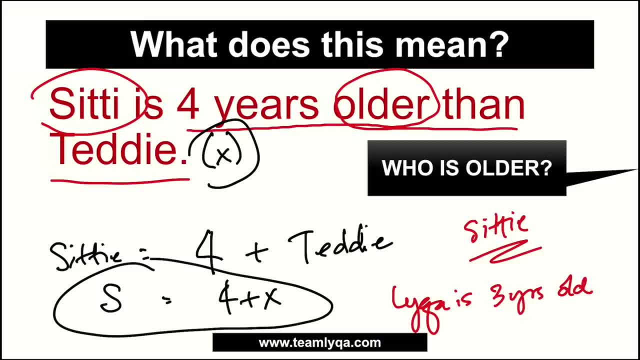 is three years older than Jana. Okay, Anong ibig sabihin yan Yung edad ko? okay, ngayon ay three plus yung edad ni Jana. Now, bakit dito ko idadagdagan sa kay Jana, Kasi nga siya yung mas bata. Okay, Kasi yung edad ko, dahil ako ay mas matanda, ay three plus yung edad niya. Kasi, kung dito ko dadagdag kay like kay, yung plus three. 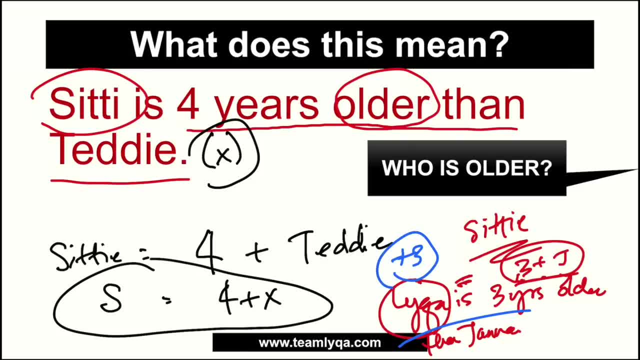 okay, hindi na totoo yung statement. Kasi kung edad ko ay dadagdagan ko pa ng tatlo, mas matanda na si Jana sa akin diba, Kasi ano magiging age ko plus three pa? eh currently mas matanda na nga ako sa kanya. eh Dadagdagan ko pa ng tatlo di di hamak na mas matanda pa yung age na yun kesa sa kanya. So again, very important na skill yung tagalugin or tagalize yung mga statements, para mas maintindihan niyo siya at mas matranslate mo siya into an equation. Again ask yourself: sino ba talaga mas matanda? 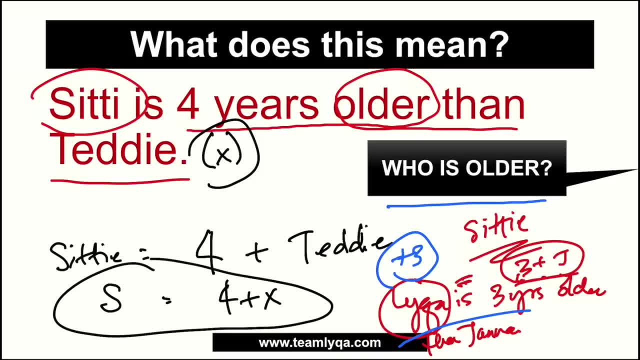 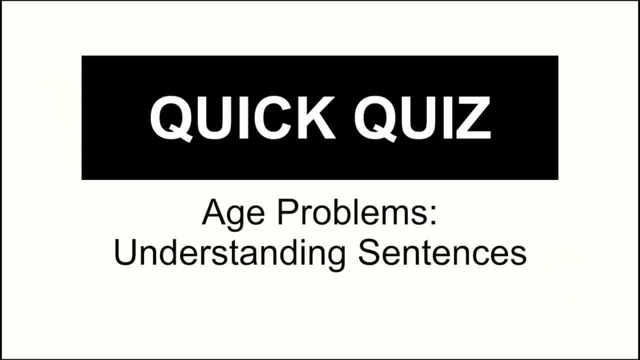 Kasi yun yung magdedetermine kung sino ang imumultiply mo, sino ang ia-add mo, sino ang isusubtractan mo na age. Okay, Now let's try this quick quiz. Okay, I'm going to give you five statements and I'm going to give you time para intindihin silang. maigi at isulat yung equation, So, parang kanina diba, si T is equal to four plus X, with X being yung age ni Teddy. Now, paano mo siya maisusulat, Paano mo siya hihimayin? And I'm going to give you a few minutes. 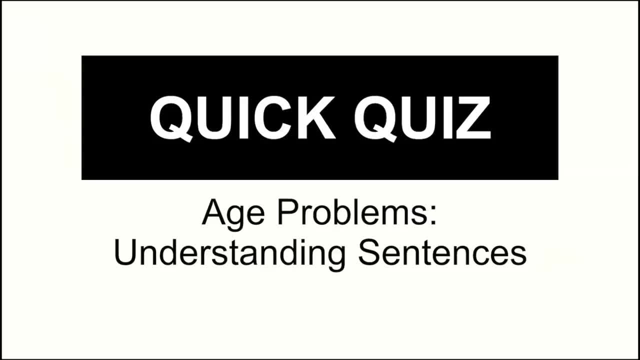 After this medyo matagal-tagal para ma-dissect yung maigi, isulat nyo lang lahat, and then we'll solve it together after. Okay. So if you're ready with your pen and paper, your timer starts now. 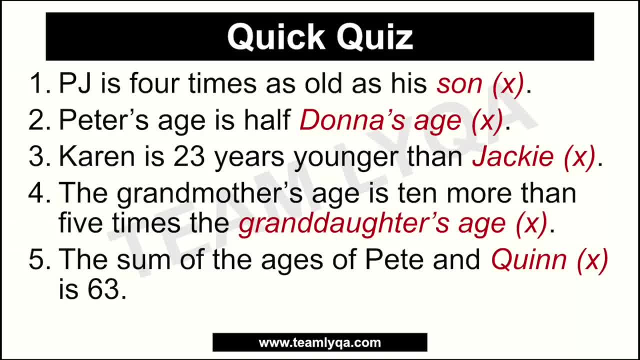 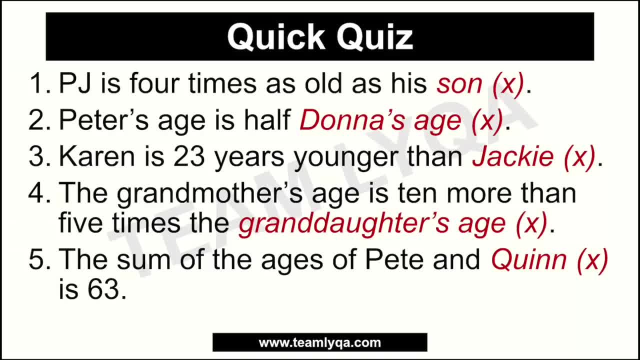 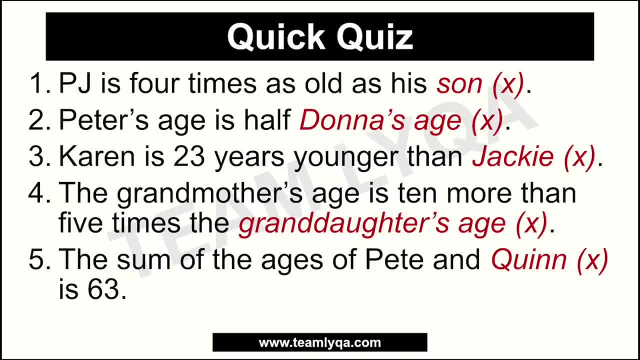 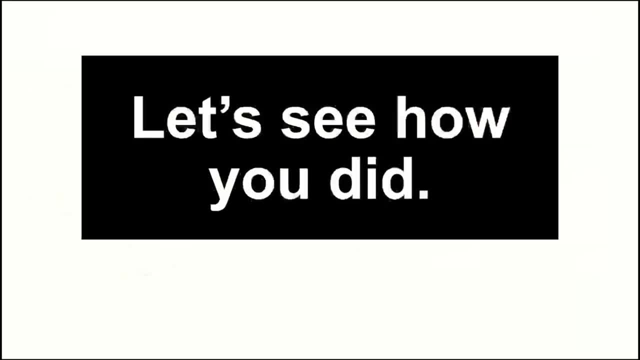 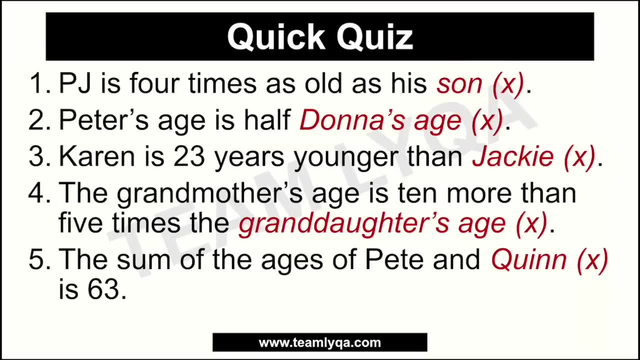 Okay. So if you're ready with your pen and paper, your timer starts now. Okay, let's see how you did So. again, we have five statements here. Yung mga nakapula sila, yung mga ex in this situation. Okay, Para lang, hindi naman kailangan isulat ng buo yung mga pangalan or kung ano yung kanilang relationship. no, So yun yung gagawin natin. mga ex. 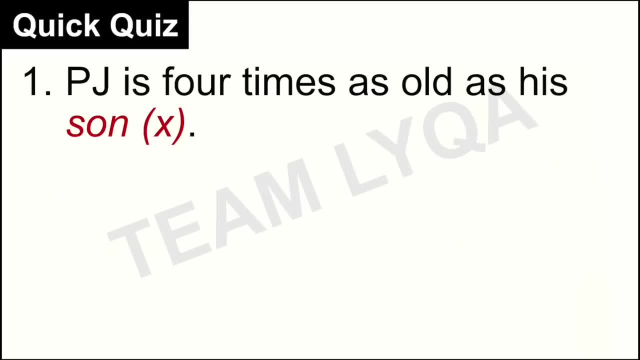 Now isa-isahin muna natin sila son. so sa tagalog si pj daw ang edad niya ay four times nung kanyang son. again, sinong mas matanda, syempre si pj kasi sya yung father. eh, no, alam ka namang mas matanda yung son kesa sa father. 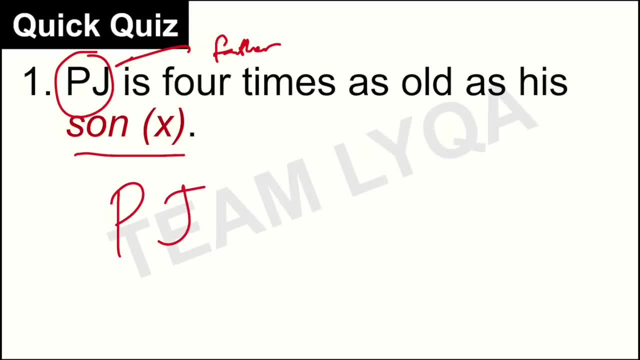 so ibig sabihin no ng age ni pj is. and again, with our equation construction, ang ibig sabihin ang is ay equal four times nung edad ng kanyang son. okay, or pj is equal to four x yung age ni pj. 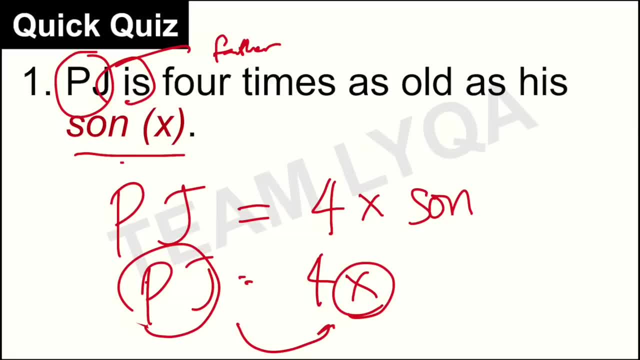 ay four x, kasi yung x is yung edad nung kanyang son. now again, kung hindi nyo pa napapanood yung aking video on equation construction, ililink ko na lang din sya dito sa taas para makapag catch. 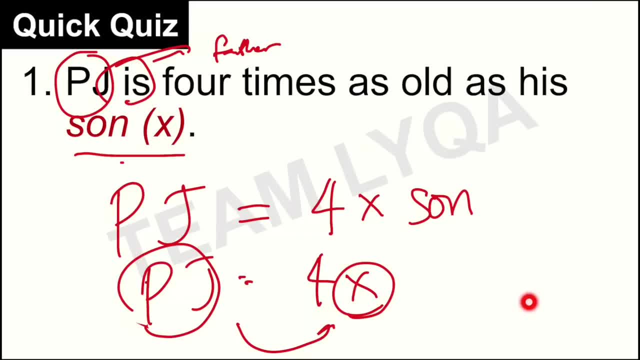 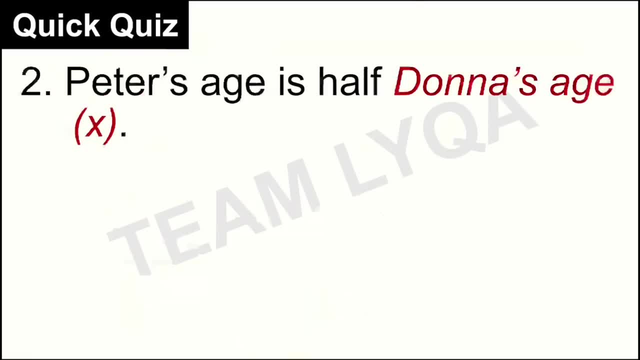 up kayo marami dun sa mga diniscuss, ko dun ang importante sa lesson na ito. kung hindi nyo pa yung napapanood, panoorin nyo muna. okay. next ililevel up. natin sabi: peter's age is half donna's age. okay, so age daw ni peter. 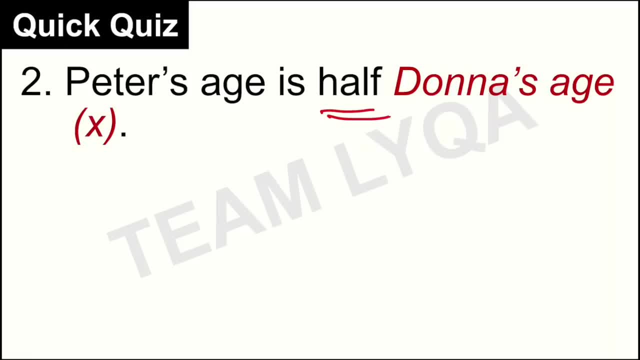 ay kalahati ng age ni donna. okay, so age ni peter is so again equal. ang ibig sabihin yan half ang half is one half, so one half of donna's age, which is our x. so peter's age is equal to one half. x with donna's age is one half, so peter's age is equal to one half. x with donna's age is. 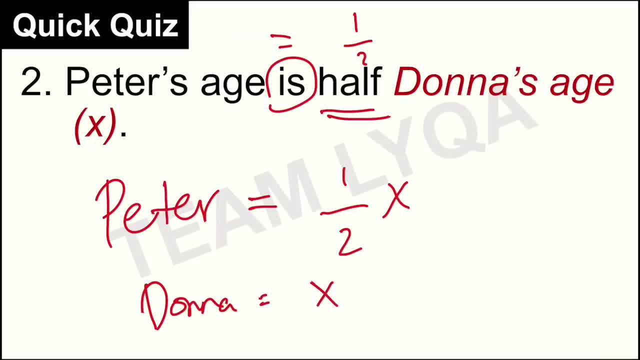 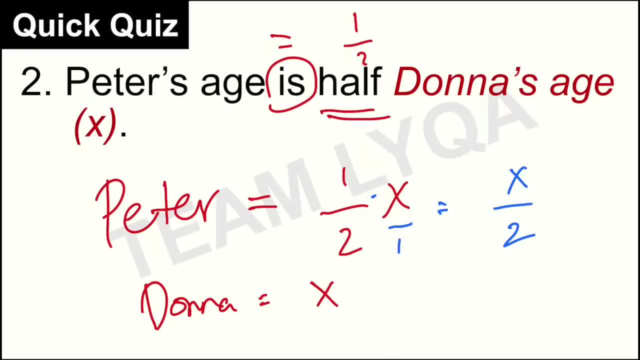 is over 1 din sya. Hindi lang natin sinusulat itong part na ito. Kung hindi nyo pa naiintindihan yung multiplication of fractions, this is not the best lesson for you, Kasi you have to. 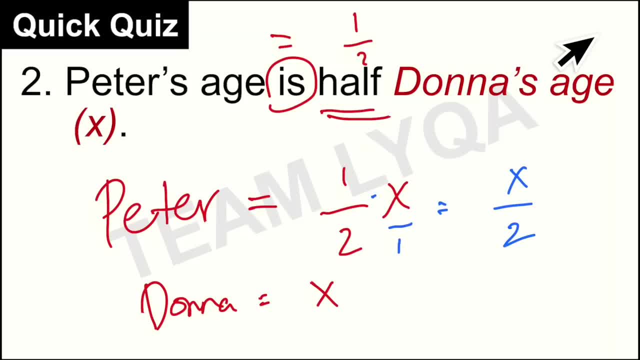 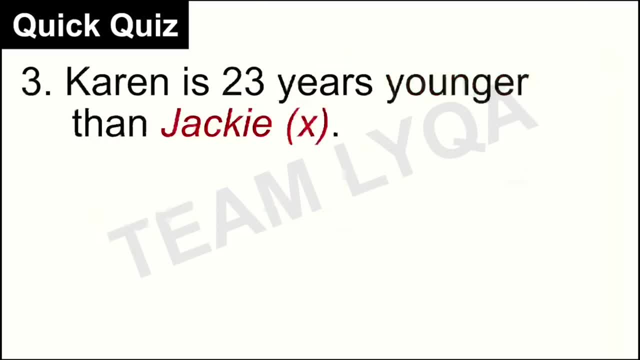 go back to your fundamentals para masolve nyo sya using yung equation natin. So if you haven't seen my fraction series, ilink ko na lang din sa taas. Now, dito tayo sa number 3.. Karen is 23 years younger. 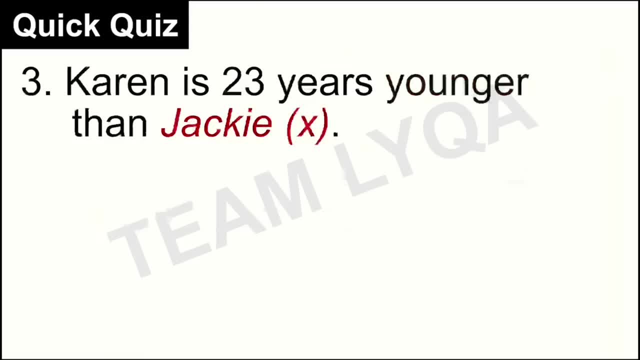 than Jackie. This is trickier than the other one, Kasi kanina older lang. eh Now, pag sinabi natin 23 years younger, Tagalogin natin: si Karen daw is 23 years younger than Jackie, So sinong mas matanda sa kanila. 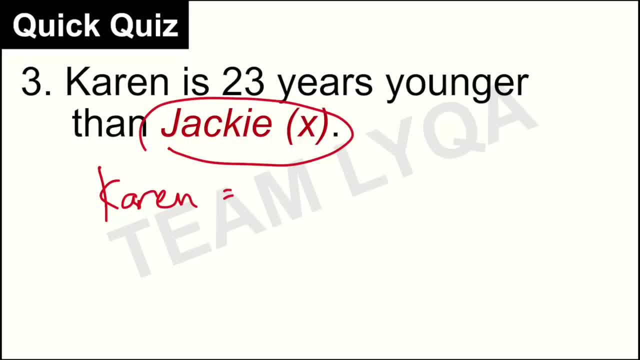 Who is older, Ang mas matanda would be Jackie. Bakit? Kasi nga si Karen ay younger kesa kay Jackie, So ibig sabihin yung edad ni Jackie, yun ang babawasan ko ng 23 para lumabas yung edad ni. 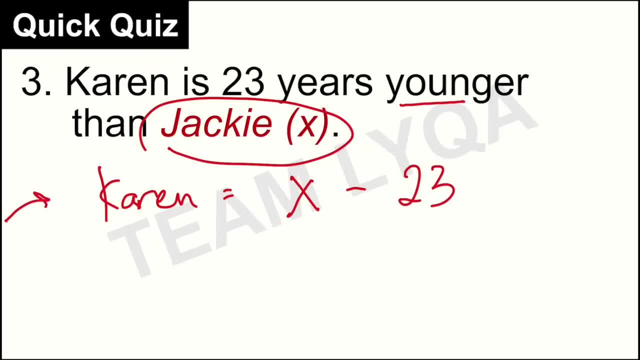 Karen. Okay, Again, using yung aking example, kanina, which is Jana, Si Jana, kasi is 3 years younger than me. Okay, Para makuha ko yung edad ni Jana, kukunin ko yung edad ko. 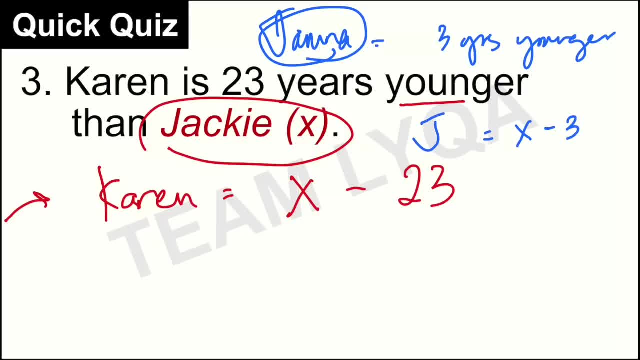 which will be x, babawasan ko siya ng 3.. Ito yung magiging edad ni Jana. Okay, Kasi lagi siyang mas bata sa akin. Ganun din yung idea dito. Now a common mistake. 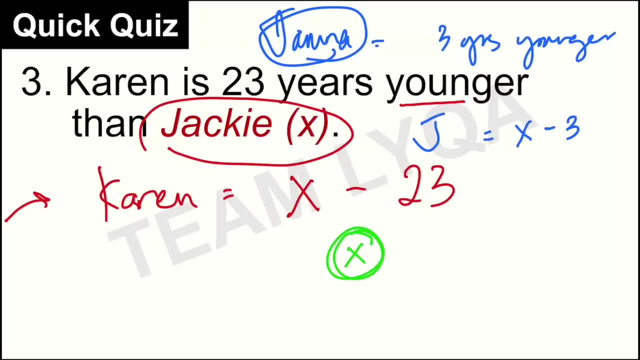 okay, dito sa tanong na to again. and this is wrong: ha, ang mali na pagkakasulad dyan would be either si yung edad ni Karen, yun ang babawasan ng 23, tas yung edad ni Jackie. 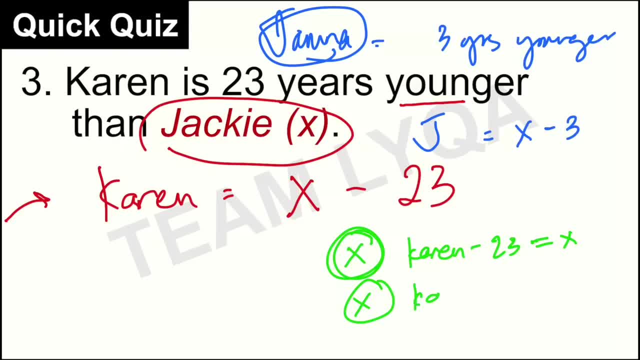 Yung iba mali din ito ha ginagawa nila is yung edad ni Karen is equal to 23 minus x. Okay, This is also wrong, kasi sa subtraction very important yung placement, kung alin. 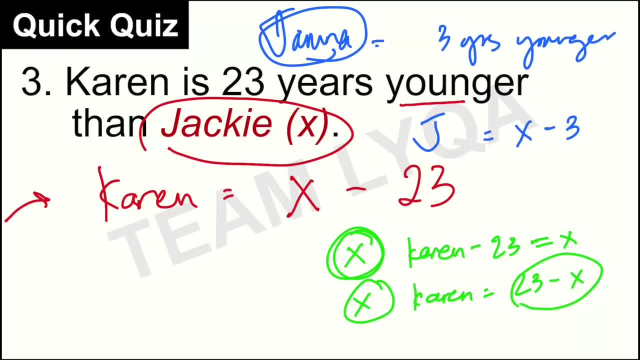 ang nauuna at ang nahuhuli. Okay, Pag ganito yung pagkakasulad mo, mali yung magiging sagot. So again, very important to think of it this way. Okay, Bakit. 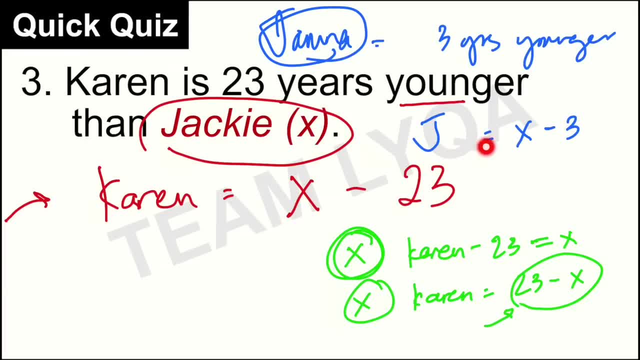 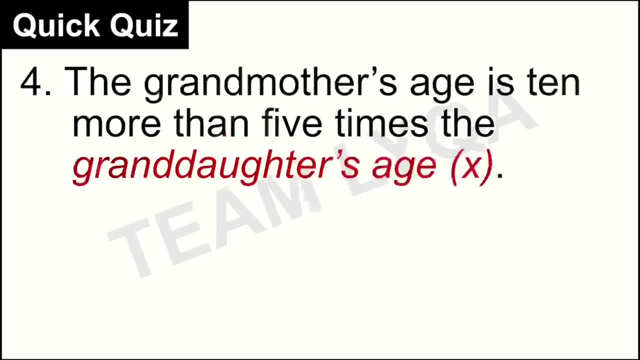 Kasi yung edad ni Jackie, pag binawasan ko ng 23,, lalabas yung edad ni Karen. Okay, Number 4.. The grandmother's age is 10, more than 5 times the granddaughter's age. Okay, Now, mukhang. 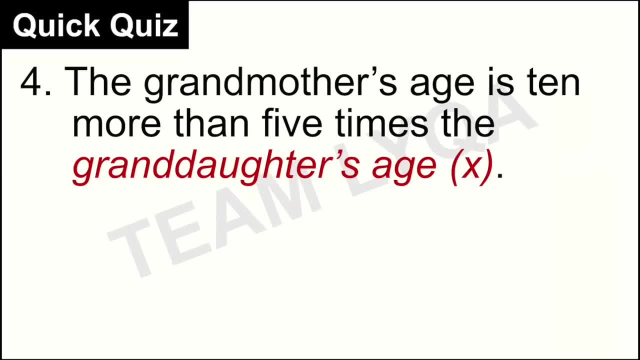 komplikado. Hihimayin lang natin again using yung ating concept ng equation construction: Yung grandmother's age, so grandmother's age is. so again equal siya 10 more than Ang, more than means addition. 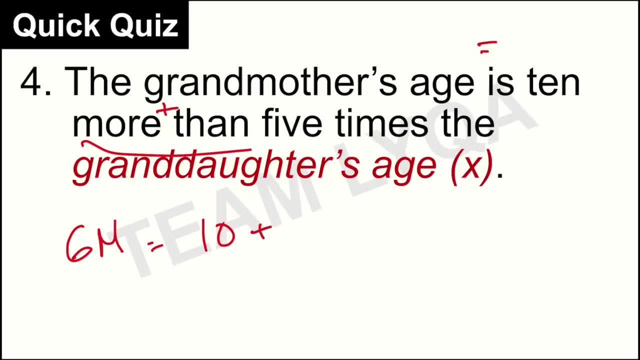 kasi sampo higit pa kaysa dun sa 5 times. Ang 5 times is 5 times nung granddaughter's age. Okay, So ibig sabihin nun, yung edad ng grandmother is equal to 10 plus. 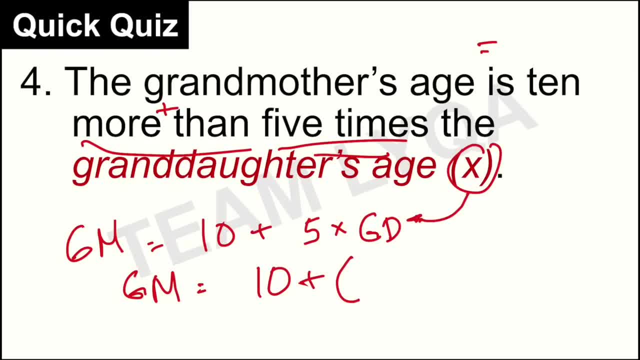 and then again, dahil yung x natin ngayon ay yung age ng granddaughter, that would be 5. x. Okay Yan, yung pagkakasulat niyan. Now, an alternate way of writing this would be yung: 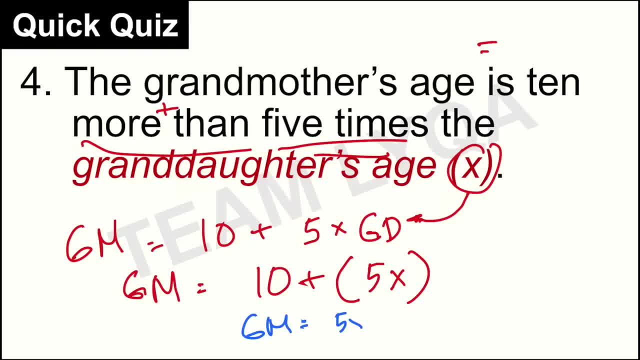 age ni grandmother is equal to 5x plus 10.. Pwede mo rin siyang isulat, na ganyan. Bakit Kasi, whether unahin mo yung 10 sa 5x o unahin mo yung 5x sa 10,, wala namang? 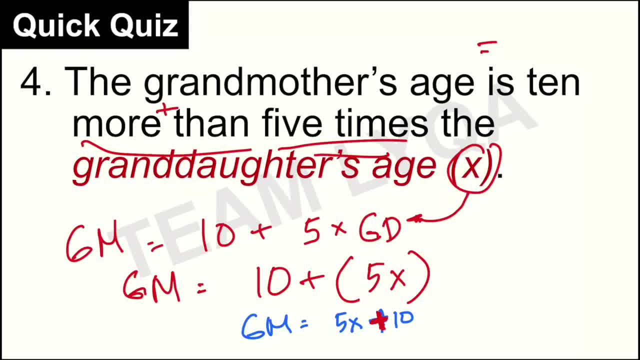 magbabago dun sa magiging sagot. Pareho lang din yan, Okay. So whether sinulat niyo yung ganyan o ganyan, pareho namang tama yan. Now, an example would be this: no Kunyari. 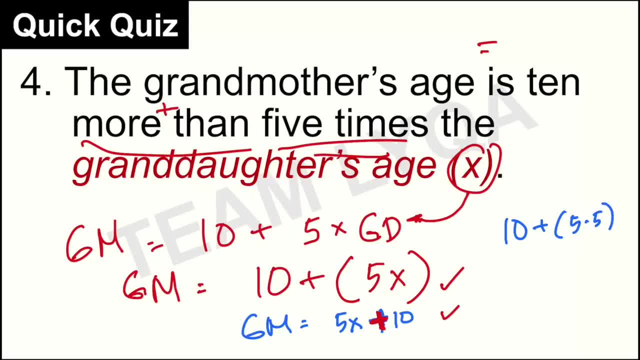 10 plus kunyari lang ha 5 times 5,. this is 10, and, using PEMDAS, 10 plus 25.. This is equal to 35. Now, kahit isulat ko siya na 5 times 5,. 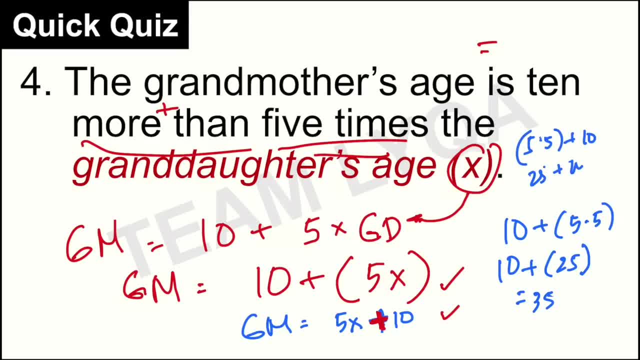 yung quantity na yan plus 10,, 25 plus 10, pareho, lang naman na 35 ang lalabas. Okay, The only time na importante yung placement ay sa subtraction at division, kasi pag ano yung nauunat nauhuli. 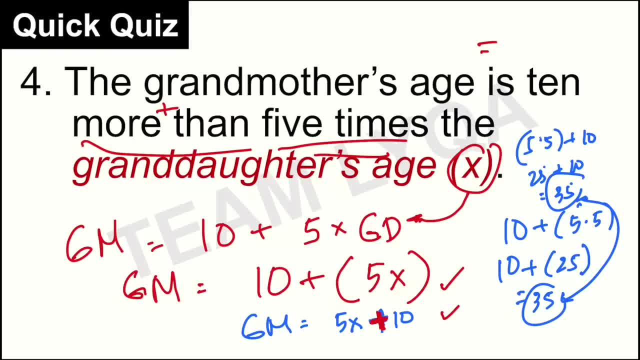 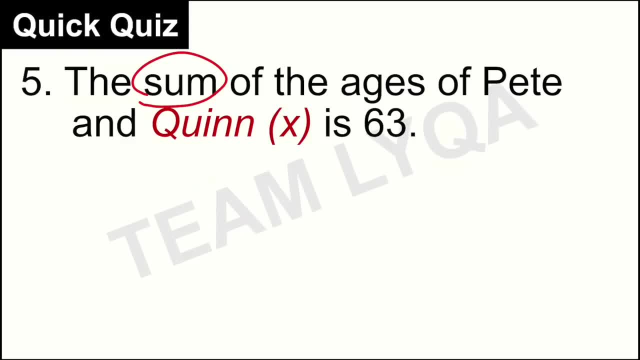 it will turn yung answer ninyo completely wrong. Number 5, the sum of the ages of Pete and Quinn is 63. Now ano ang implication nito? Okay, Ang sabi natin yung sum daw ng ages nila Pete. 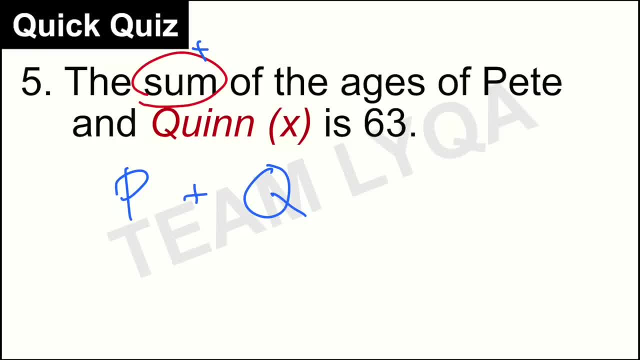 at Quinn, ibig sabihin ng sum. ibig sabihin yung pitag-add mo sila is equal to 63.. So ganyan yan. Pero dahil ang edad ni Quinn is our X sa problem na ito gagawin. 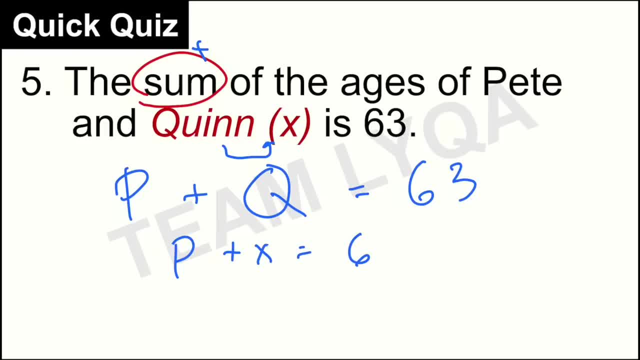 natin yung age ni Pete plus X is equal to 63.. So ang hinahanap lang natin na edad ni Pete, okay, kailangan natin siyang iwan sa isang side, So P is equal. 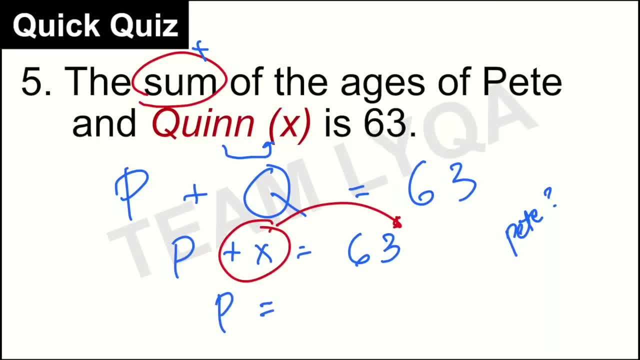 to itatranspose natin yung plus X, nilipat natin sa kabila, At pag nilipat mo siya sa kabila magiging minus siya. So that would be 63 minus X. So si Pete ay 63 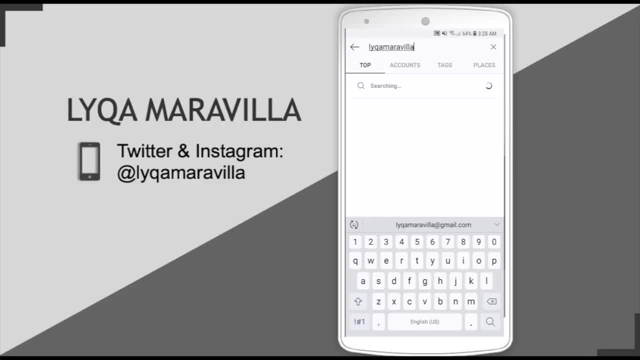 minus X. Alright, I hope you got that right. If you didn't, that's okay. I'll be posting more examples on my Instagram account. So if you don't follow me yet, follow me at Laika Maravillo for yung quick quiz. function natin. 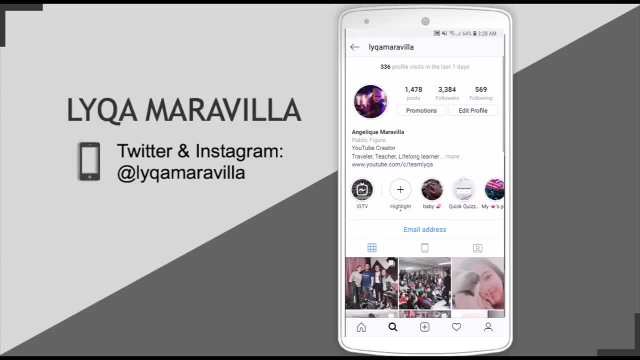 Sa Instagram story you can see yung mga multiple choice questions At pwede kayo mag-participate dun to find out if you get it right. It's a great way din for me to know kung ano lessons yung kailangan.